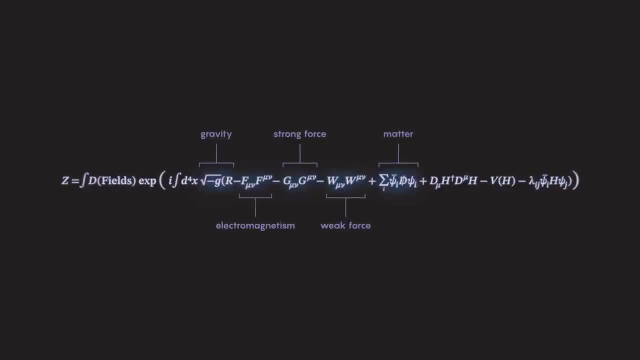 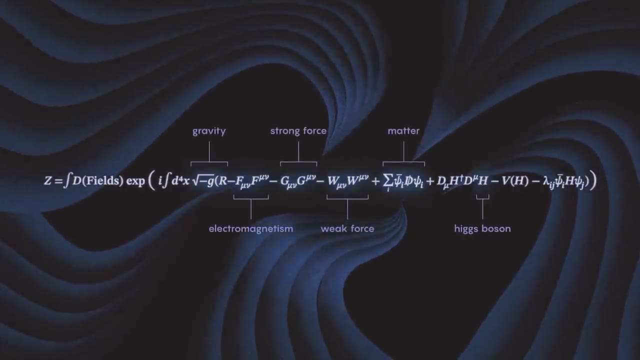 of thousands of experiments, in some cases with an accuracy that is unprecedented in science. It is, by any measure, the most successful scientific theory of all time, And yet, for something so extraordinary, we give it a rubbish name. We call it the Standard Model. 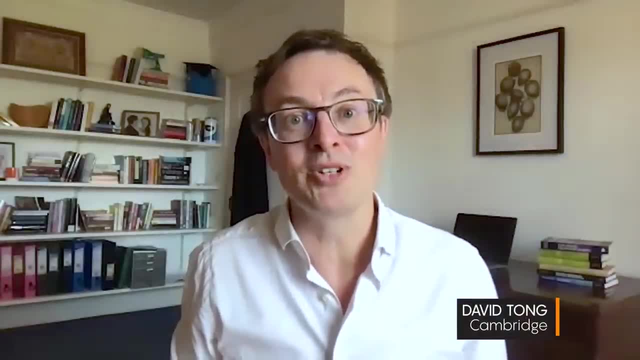 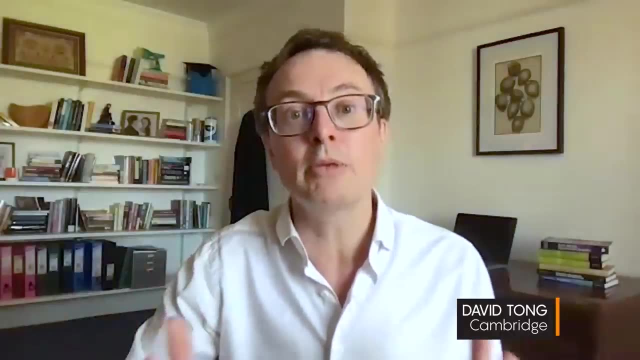 I'm David Tong, a theoretical physicist at the University of Cambridge, and in this video we're going to build the Standard Model piece by piece. I hope that by the end you'll have some intuition for how the different parts fit together to create the 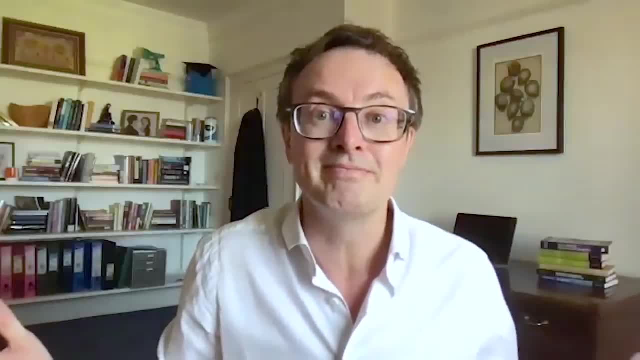 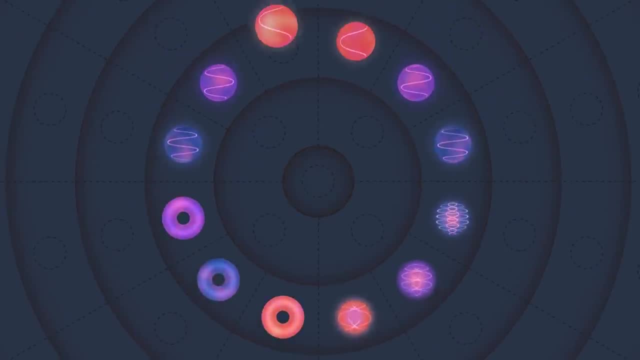 fundamental building blocks of our universe. This is the Standard Model. It describes how everything in the universe is made of 12 different types of matter, particles interacting with three forces, all bound together by a rather special particle called the Higgs Boson. 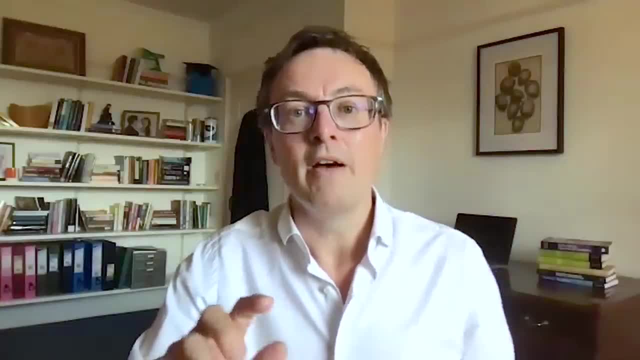 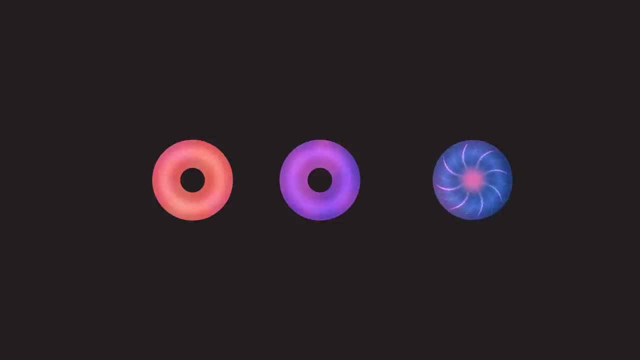 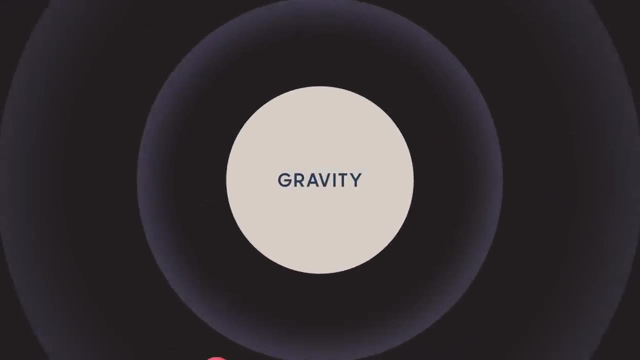 Before we get going, some caveats. First, I said three forces. Well, there are actually four fundamental forces at play in the universe. This means there's something missing from this picture And that something would be gravity, The most obvious force at play in the world around us, and yet in many senses, 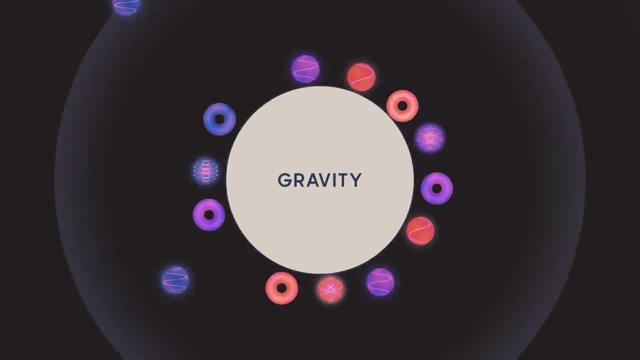 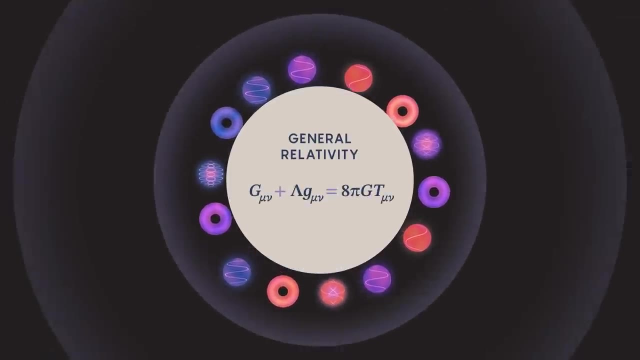 the one that we understand least. We do have a theory of gravity, a very successful theory. It was given to us by Albert Einstein and it goes by the name of the theory of gravity And it goes by the name of General Relativity. But there are two good reasons why it's not included in the 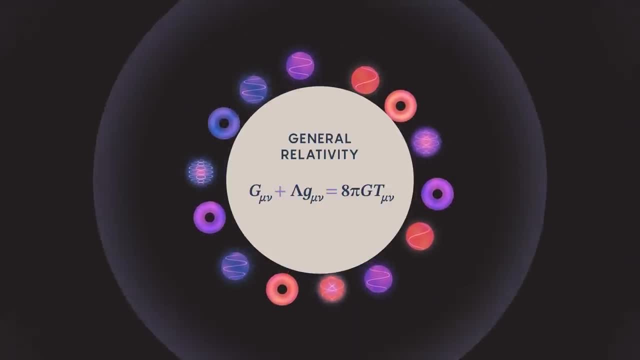 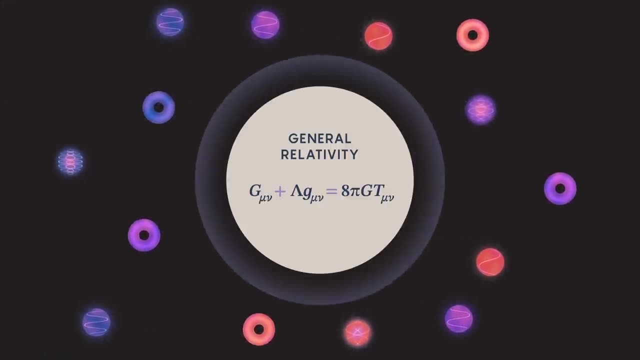 Standard Model. The first is that at the microscopic level, the force of gravity is so weak that it barely has any effect on a single subatomic particle. The second is that we don't really know how to incorporate General Relativity, which is a classical theory, into the quantum 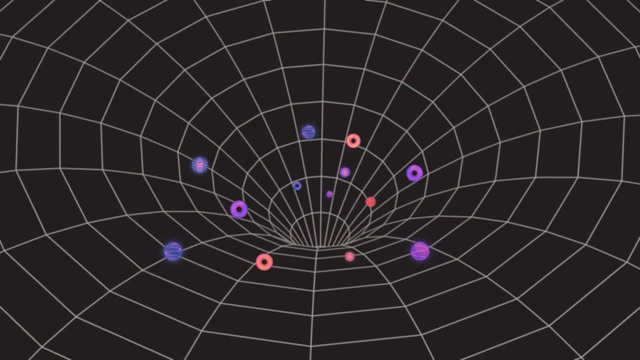 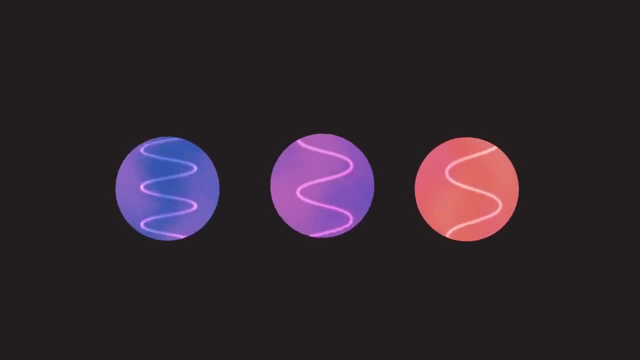 world. We have no idea how to peer into a black hole where quantum gravity effects are clearly at work. A second caveat is that the Standard Model is written in a language known as quantum field theory. This tells us that matter at the fundamental level is not really made up of. 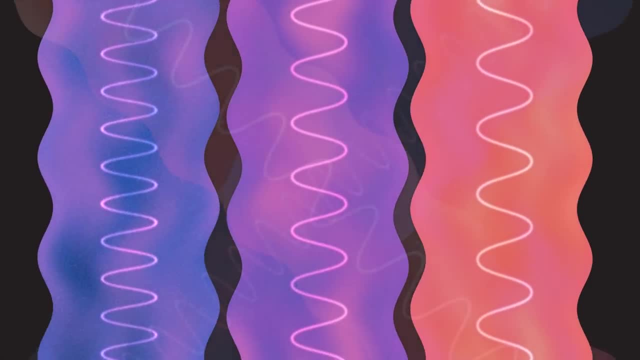 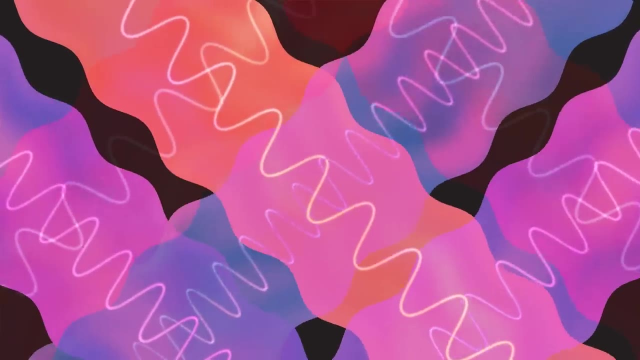 particles. Instead, it's made up of fields, Fluid-like objects, which are spread throughout all of space. These fields are engaged in an intricate, harmonious dance to a music that we call the laws of physics. The interactions between the fields produce the physical world. 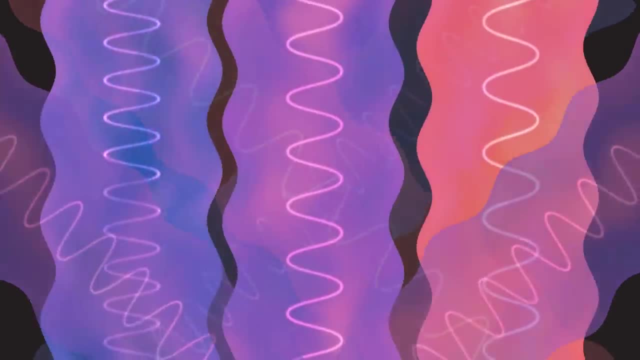 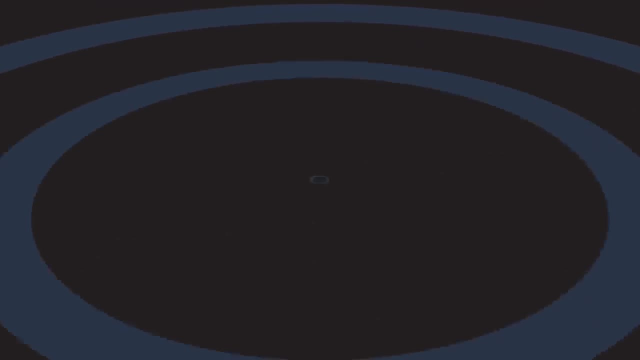 in the form of particles. To understand the Standard Model, we need to understand the laws of physics. To understand the Standard Model, it's more convenient to use the language of particles. As we build up the Standard Model, we're going to meet lots of particles with an array of names. 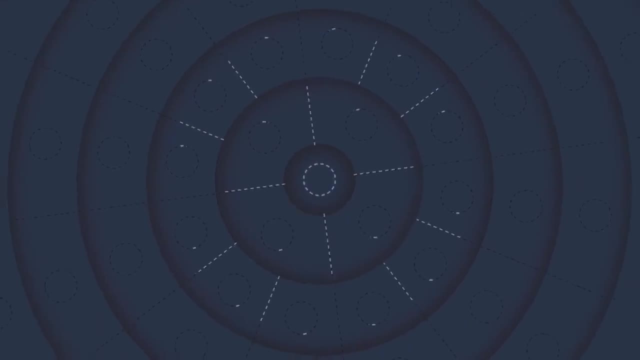 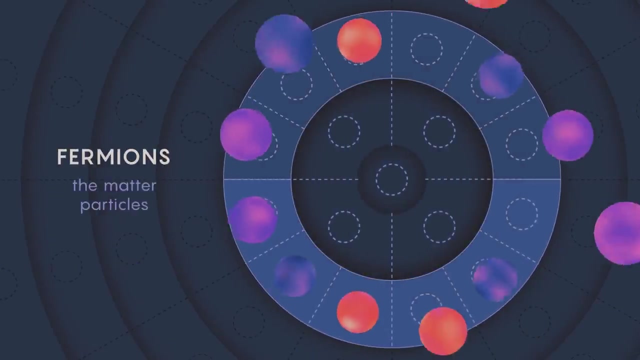 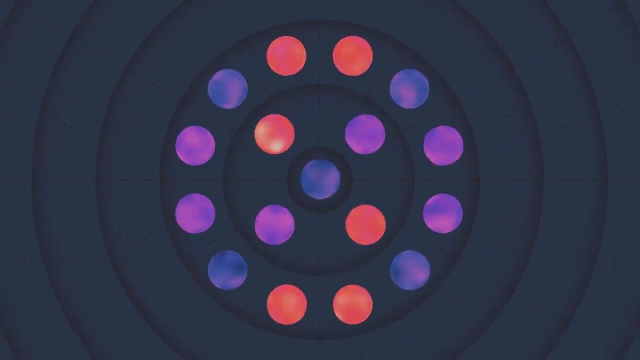 that can very quickly become bewildering, But there's one classification of particles that is by far the most important. Every particle is either a fermion, which is a matter particle, or a boson, which is a force particle. The distinction between fermions and bosons lies in 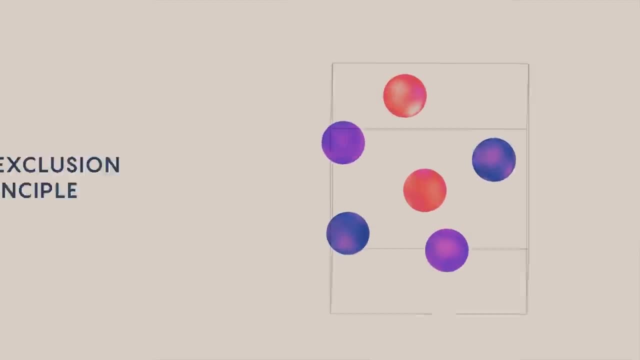 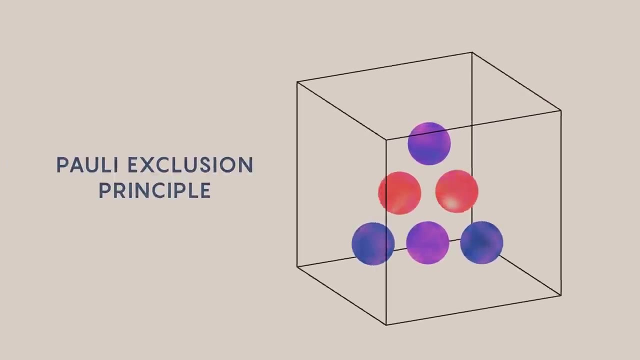 the quantum world, Fermions must obey something that we call the Pauli exclusion principle. Roughly speaking, this means that you can't put two fermions on top of each other in space. As such, these are the building blocks of matter. 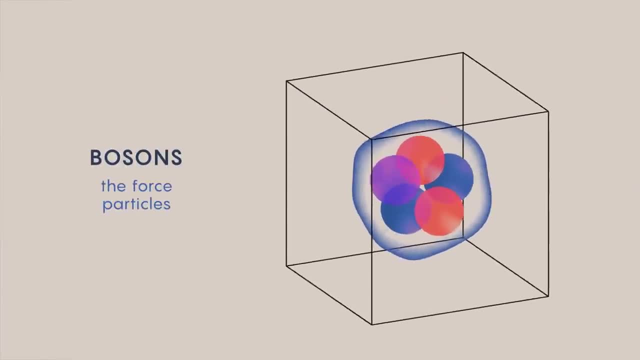 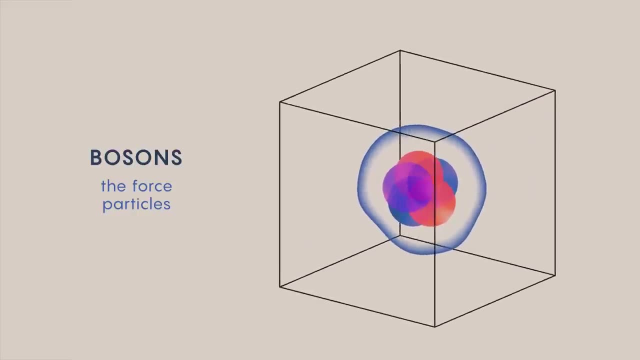 Bosons, on the other hand, can pile on top of each other as much as they want, because they're not obliged to obey the Pauli exclusion principle. Bosons are the particles that mediate various forces, and we'll talk about them much more later. 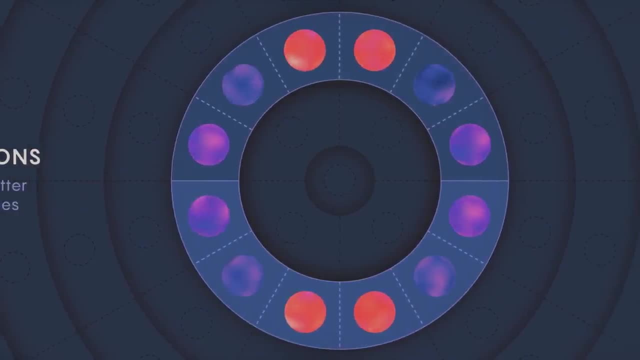 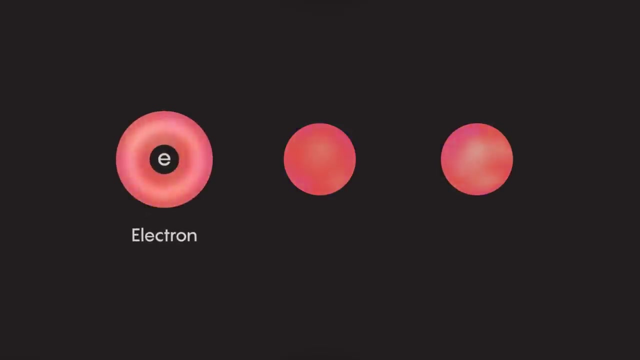 But for now, Let's start by looking at the fermions. Everything we're made of can be reduced to just three matter particles. This is the electron and two species of quarks that we call the up quark and the down quark, The familiar proton and neutron. 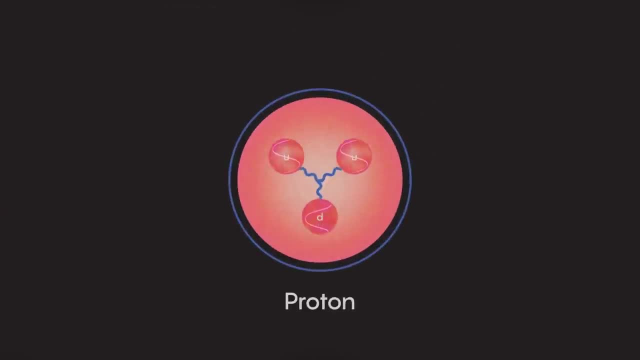 each contain three quarks. The proton has two up quarks and a down, while the neutron has two down quarks and an up. Put protons and neutrons together and you have a nucleus. Add electrons into the mix and you have an atom. Put a bunch of atoms together. 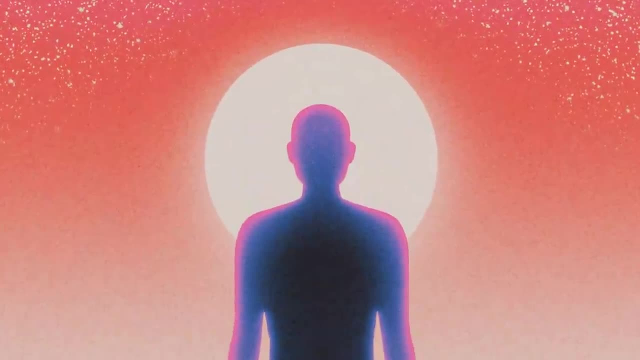 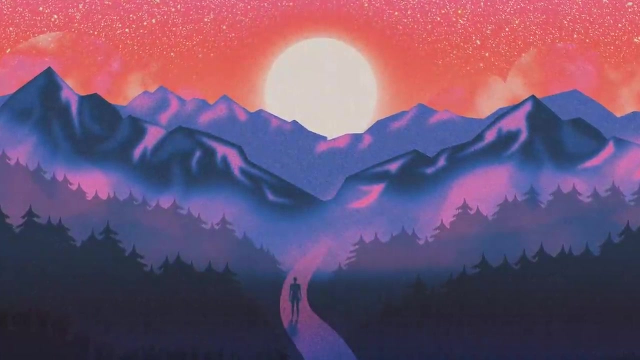 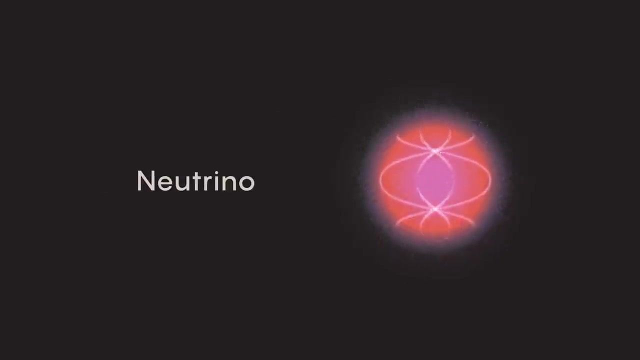 and that's what we're made of. All the beauty and complexity that we see in the world around us can be traced to the same collection of three particles rearranged over and over in different combinations. Next comes the fourth type of matter particle. It's called the neutrino. 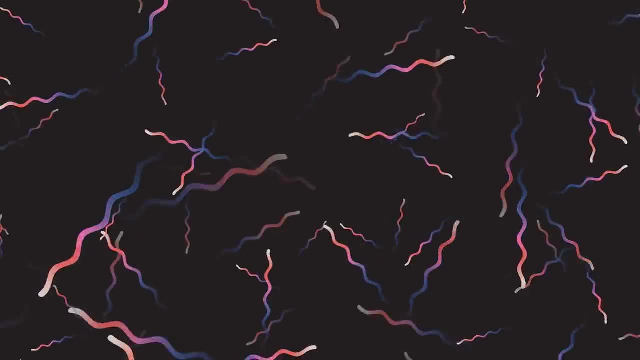 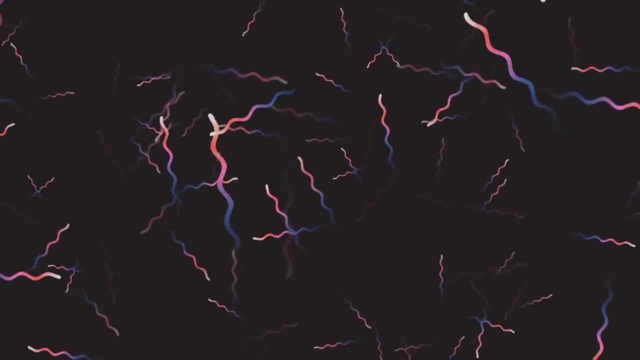 and it's not like the others. Neutrinos are extremely light and barely interact with anything else. For example, in the time it took me to say that, something like a hundred trillion neutrinos passed through your body. Most of them came from the sun, but 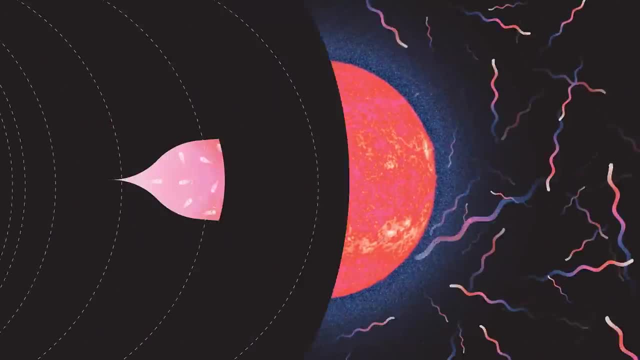 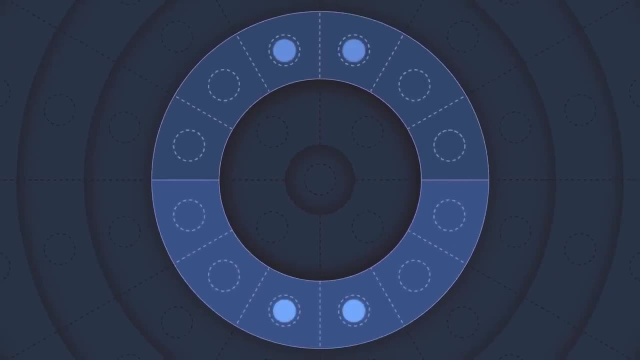 millions of them have been streaming uninterrupted through the universe since the first few seconds after the big bang. So there we have it: Four matter particles, Three that make up you, me and everyone we know, And one very peculiar cosmic ghost flowing through us all. But here's where things start to get. 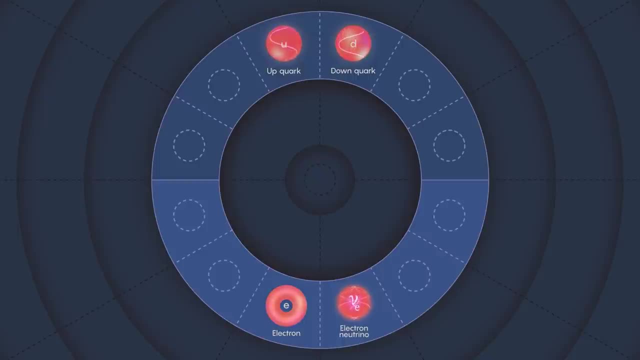 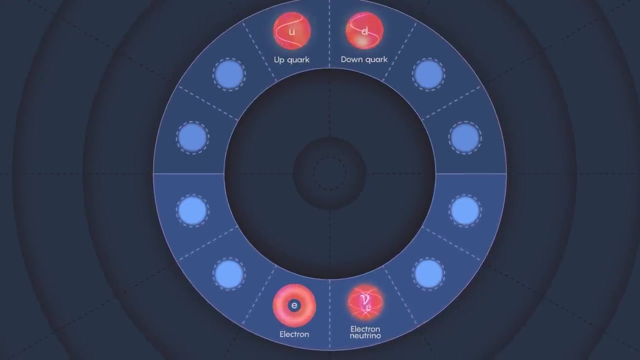 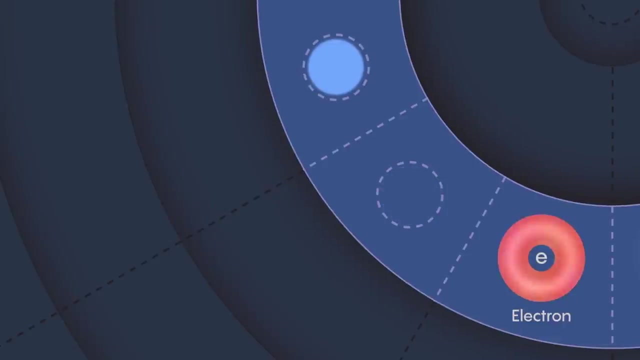 weird, Because nature didn't stop there. For reasons that we do not understand, she took this collection of four particles and made two further copies. This means that there are actually three different kinds of electron particles. In addition to the original electron that we know and love, there are particles called the muon. 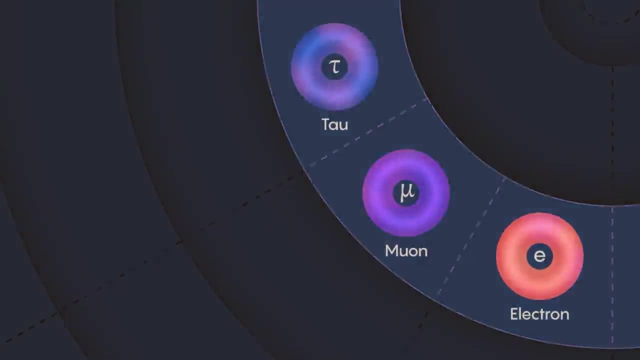 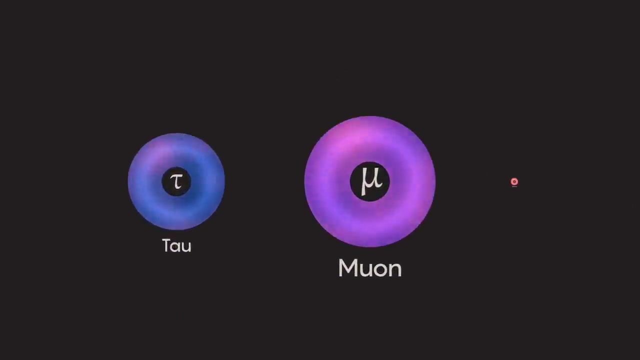 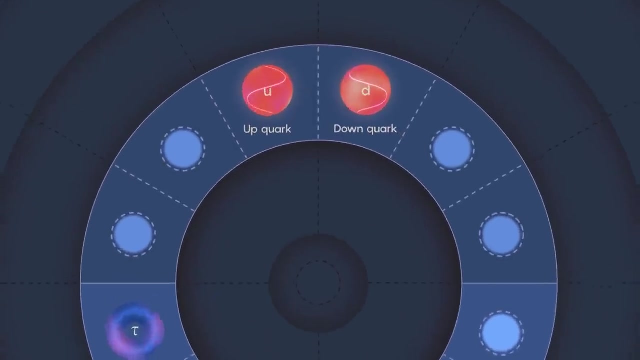 and the tau. The muon and the tau behave exactly like an electron, with one important exception: They're heavier. The muon is about 200 times heavier than the electron, The tau almost three and a half thousand times heavier. The same generational pattern then repeats for the quarks. There are two. 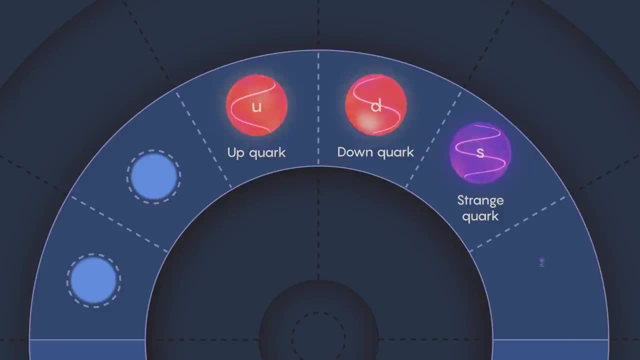 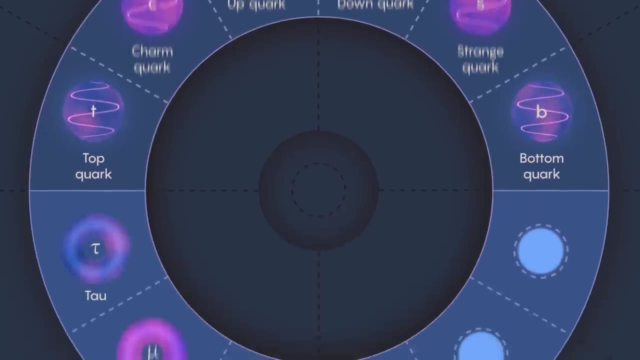 heavier versions of the down quark that we call the strange and bottom quarks, And two heavier versions of the up quark called charm and top. And then there are also two more neutrinos. We become a little bit unimaginative in our naming. 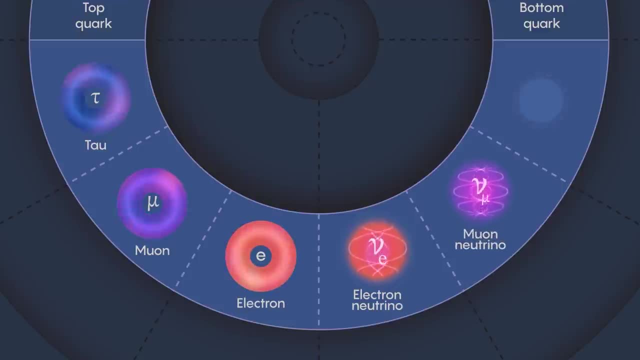 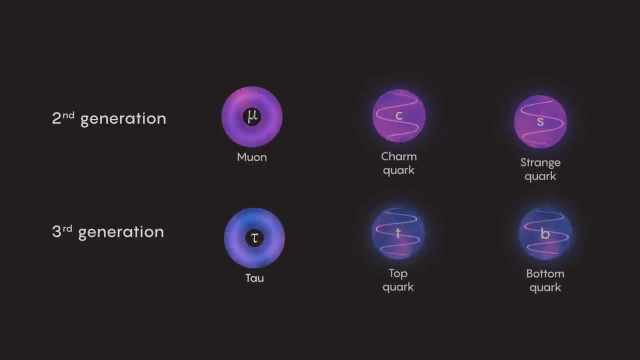 and call the full collection the electron neutrino, the muon neutrino and the tau neutrino. Now we don't see the second and third generation of particles in everyday life. We can create these heavier particles, but they're unstable, which means that they quickly decay to the first. 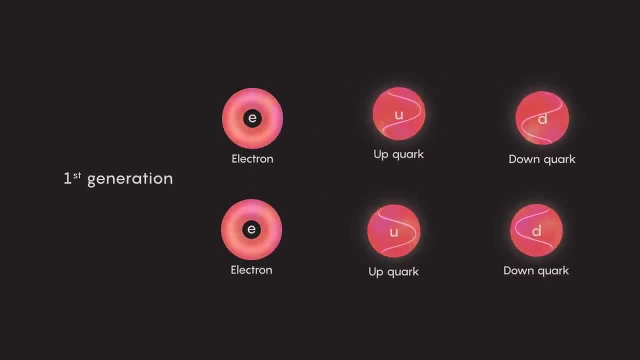 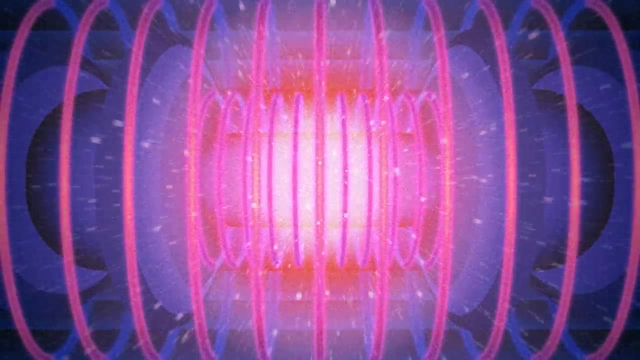 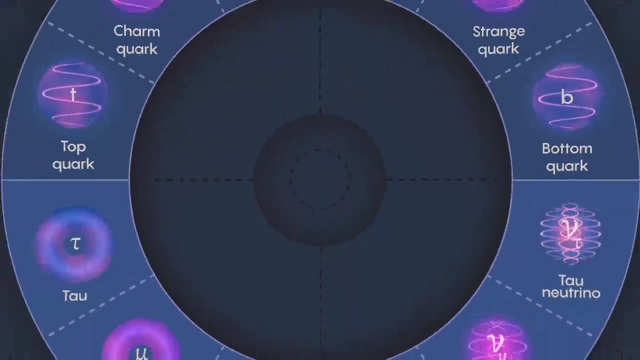 generation of particles that we're made of. Nonetheless, we know they exist. We can detect them in particle accelerators and, in many cases, we can take photographs of the tracks they leave behind. This is the collection of particles that makes up our world. 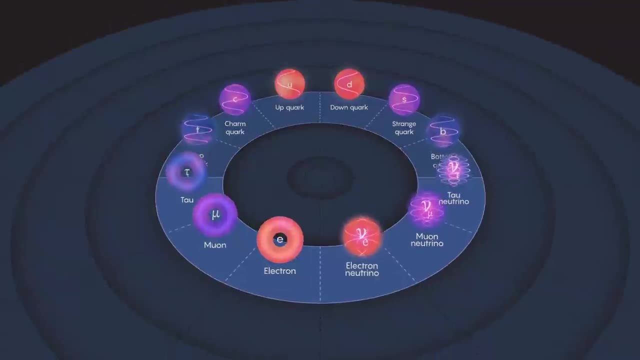 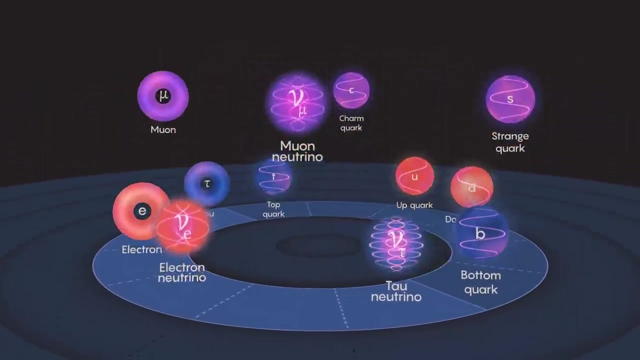 Three sets of four, And this we understand very well. In particular, we understand why particles have to come in a set of four. There's a mathematical consistency condition in the standard model that tells us you can't have one particle without the other three. 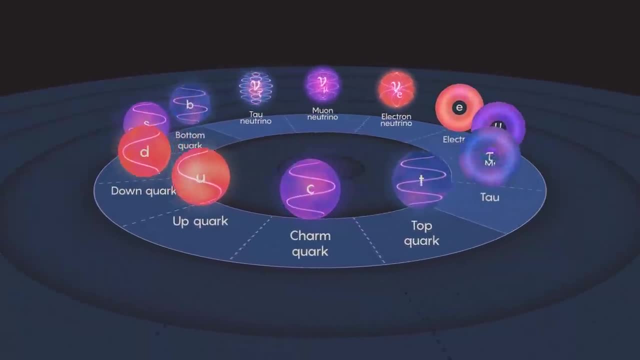 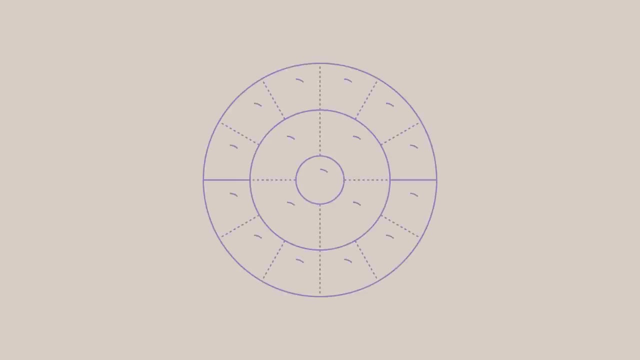 In contrast, we don't understand at all why there are three generations rather than any other number. That remains a complete mystery. There is, however, a surprising aspect of mathematical unity: here All particles are described by exactly the same equation. This equation was written down in the 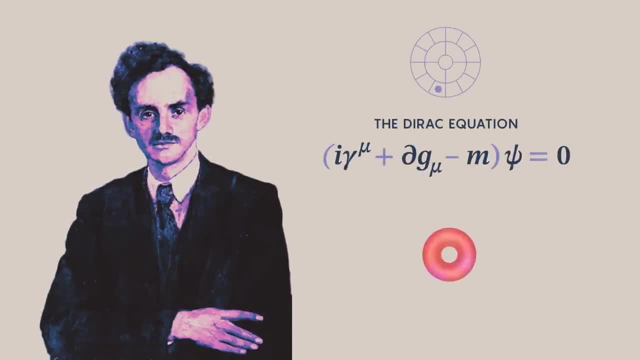 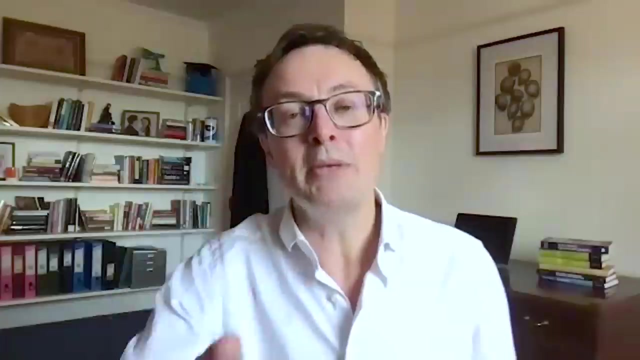 1920s by the physicist Paul Dirac, originally to describe the electron. But as we discovered more and more particles, we realized the Dirac equation, or variants of it, also describes them. So that's the stuff we're made of, But still we're missing something crucial. We're missing. 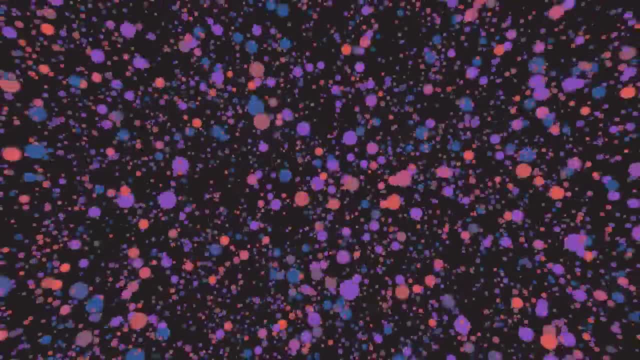 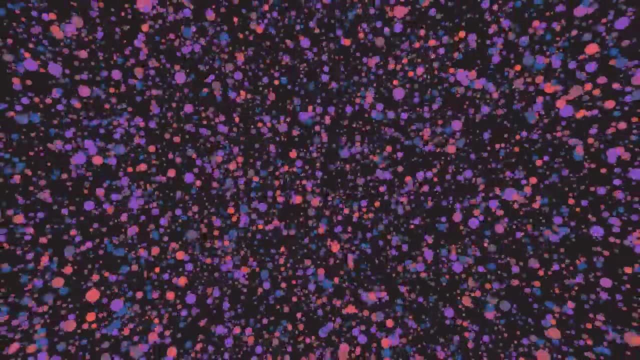 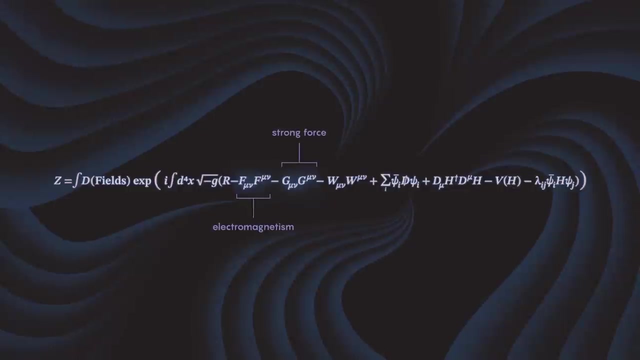 the forces. Without the forces, the universe would be boring. All the particles would wander around the cosmos like lost souls, never interacting, never doing anything interesting. There are three fundamental forces in the standard model: Electromagnetism, the strong force and the weak force. 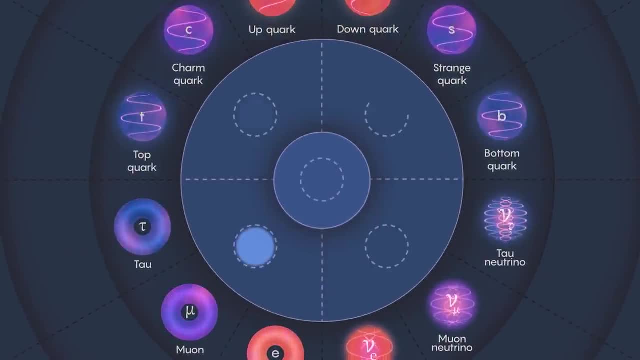 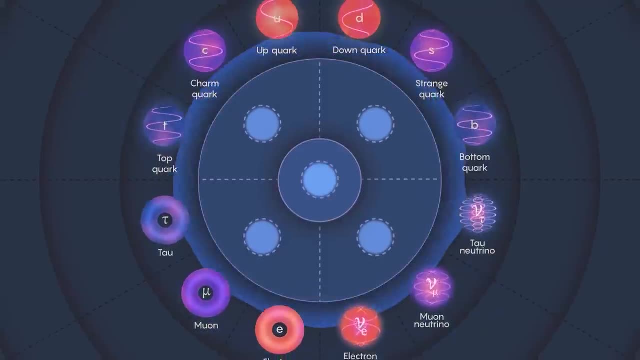 Each of these forces comes with an associated particle. These particles are what we call bosons, the other half of our particle family. Bosons are force-carrying particles. In one way of viewing things, you can think of the fermions as constantly swapping bosons between them. 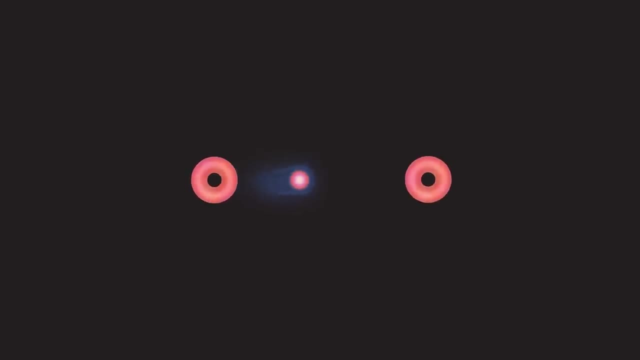 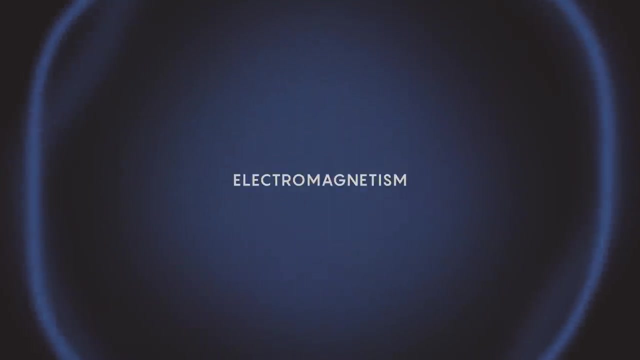 Affecting their motion and giving rise to what we call a force. Let's begin with the most familiar of these forces. Electromagnetism is responsible for the chemical properties of the elements, and we've harnessed it to create much of modern technology. 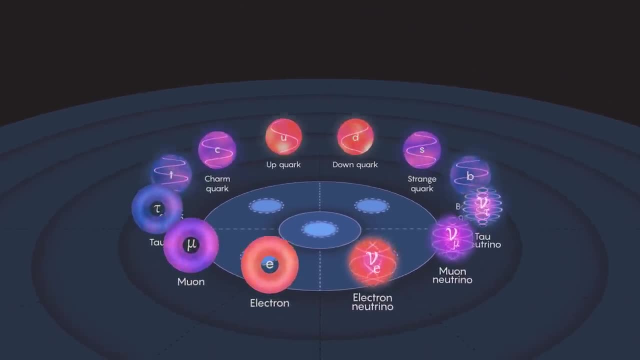 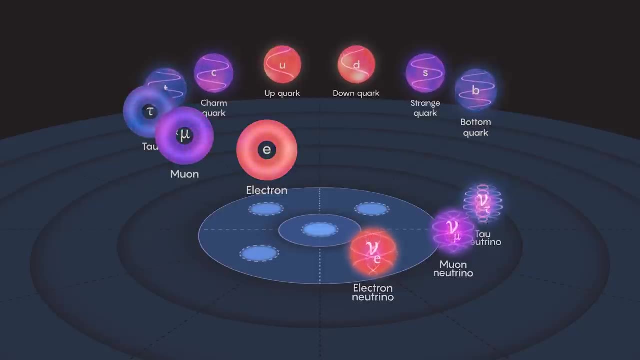 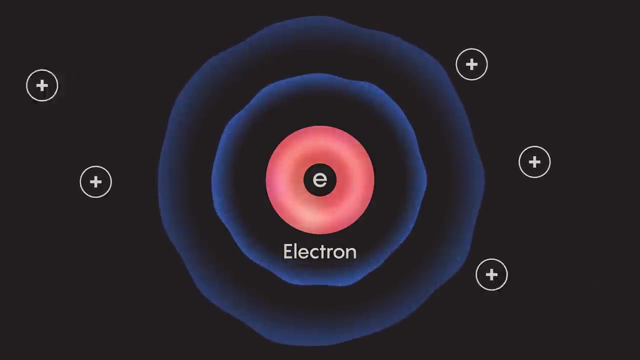 It acts on anything that carries electric charge. That means that it acts on the electron-type particles and the quarks, but not on the neutrinos, because neutrinos are electrically neutral. An electron sitting still in space will give rise to an electric field which spreads radially. 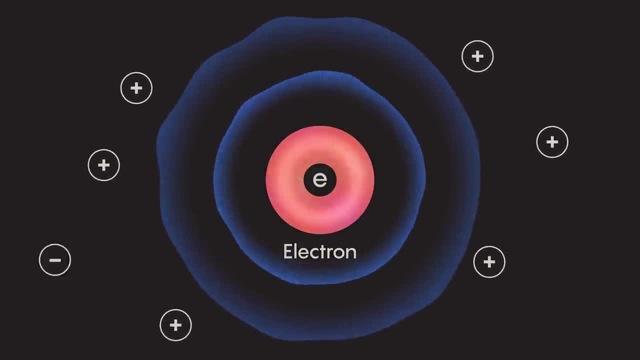 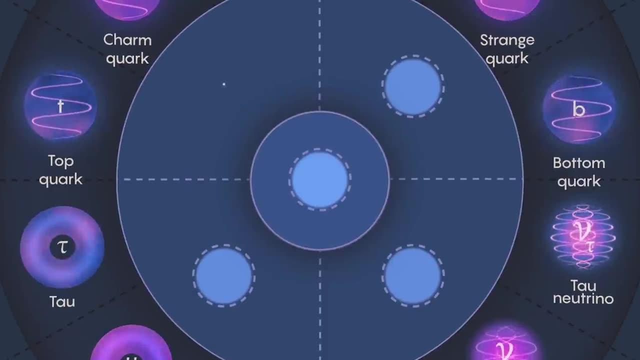 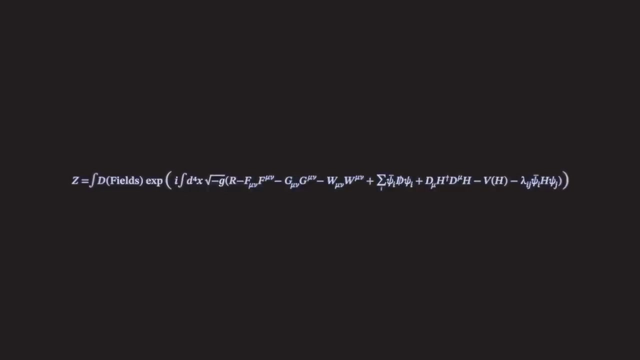 outwards and attracts or repels all other electrically charged particles in its neighbourhood. But if you look more closely at that electric field, you'll find that it's comprised of the particles of electromagnetism. These particles we call photons. Next is the strongest fundamental force in nature, aptly named, the strong force. 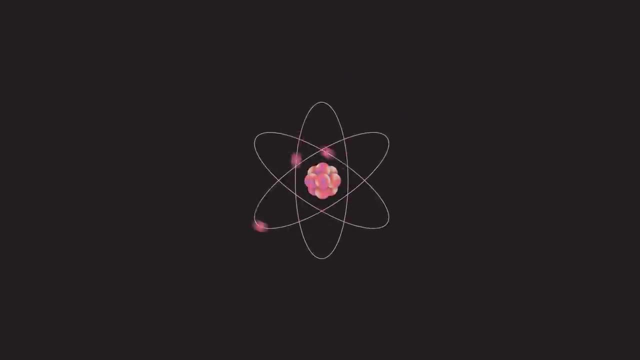 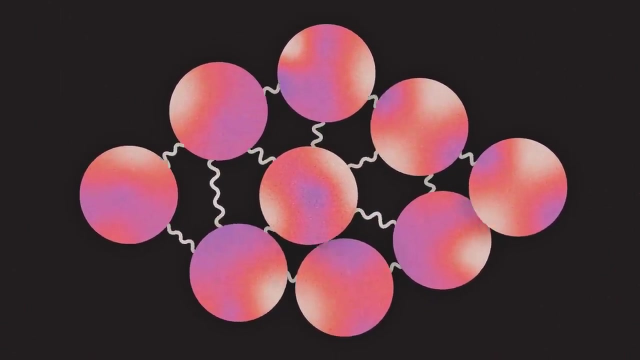 This force acts only on quarks, and some of these quarks act only on neutrinos. It acts subsequently on particles like protons and neutrons that are made of quarks. It's the strong force that holds together the nuclei of atoms. 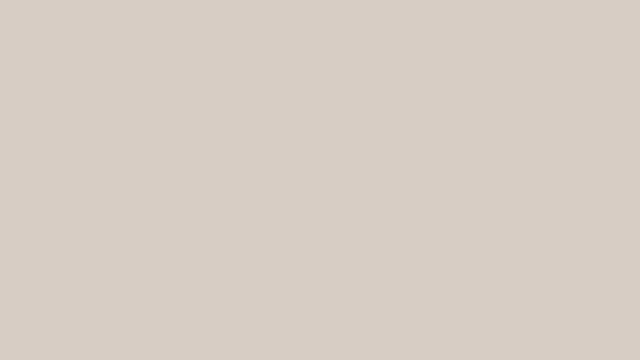 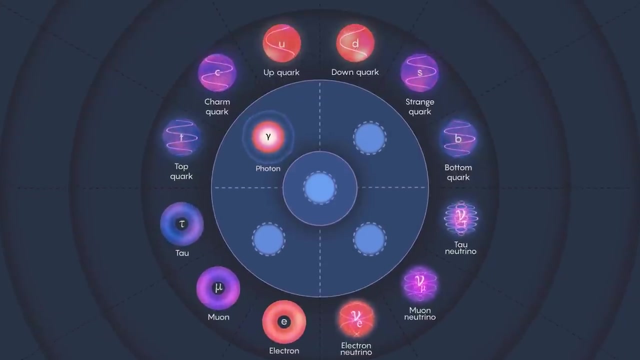 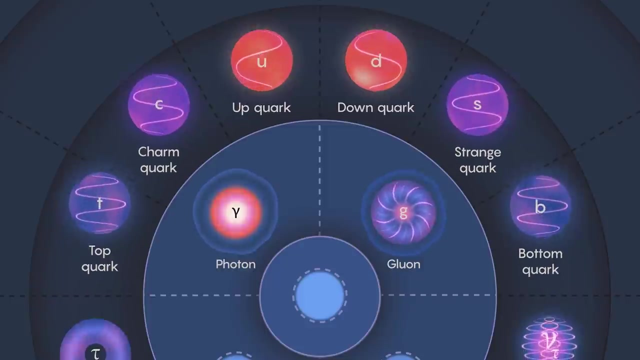 It's also this force that is responsible for nuclear fission and gives the energy that is released in an atomic explosion. Just as the photon is associated to electromagnetism, there is a particle associated to the strong force. We call it the gluon, because it literally sticks quarks together. 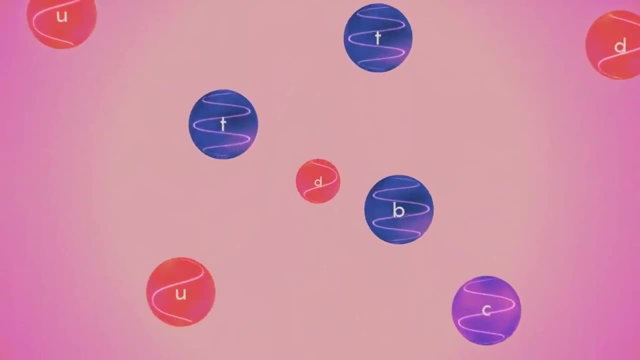 As an electron gives rise to an electric field, so a quark sitting in space will give rise to a gluon field. But now something different happens. Unlike electromagnetism, the field doesn't spread out radially. Instead, the quark produces a thin flux tube. 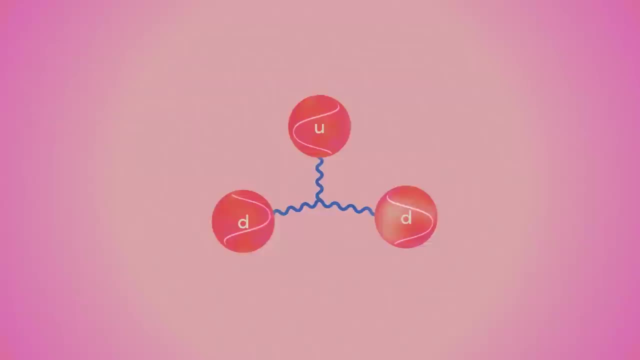 a string-like object which can only end when it finds a different kind of quark. This is what makes the strong force strong. Because the quarks are joined by a flux tube, it takes more and more energy to pull them apart. This is why we never see quarks on their own. 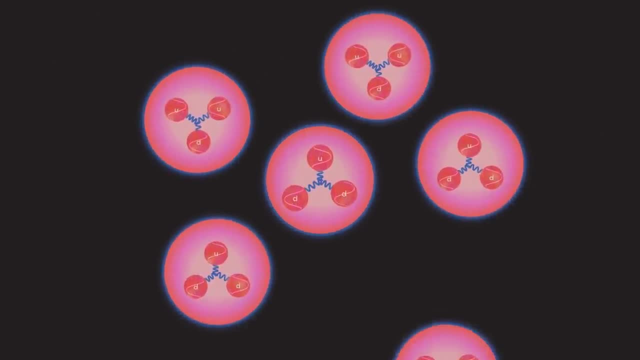 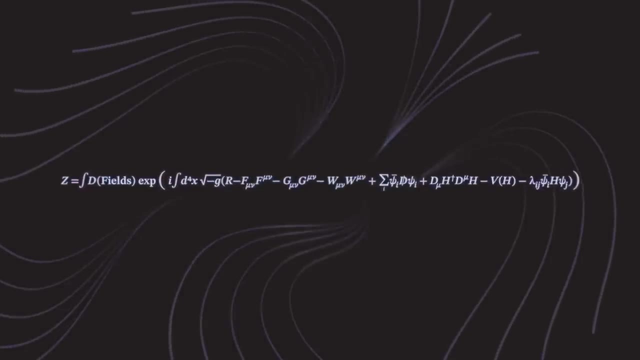 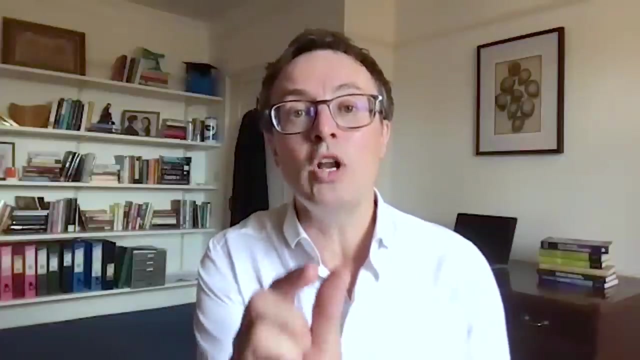 They're always bound together by the strong force inside bigger particles like protons and neutrons. The third and final force is the most intricate and subtle of them all. This is the weak force. Like the strong force, the weak force acts only on subatomic distance scales. 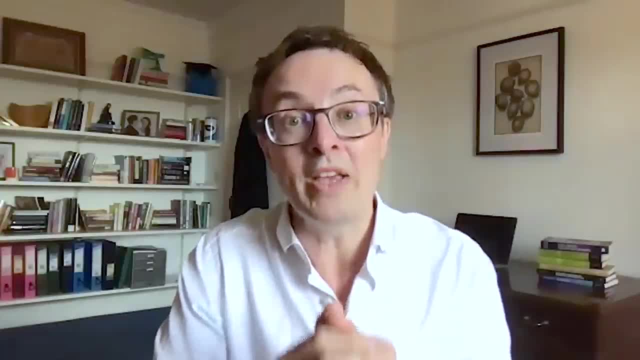 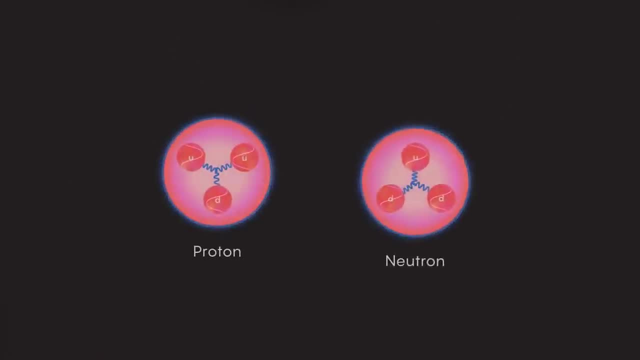 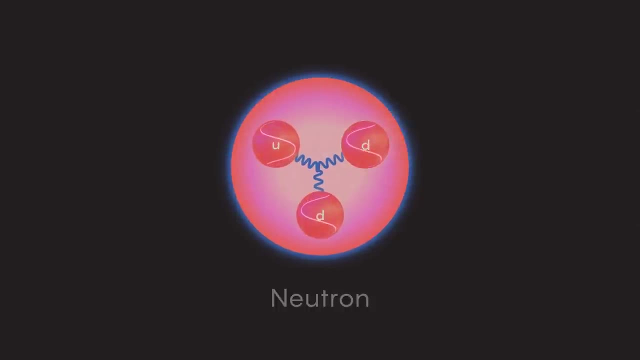 But rather than binding particles together, the weak force is all about decay. We just learned that the strong force binds quarks together to form protons and neutrons, creating the atomic nucleus. The weak force has the astonishing ability to allow quarks to switch their identity. 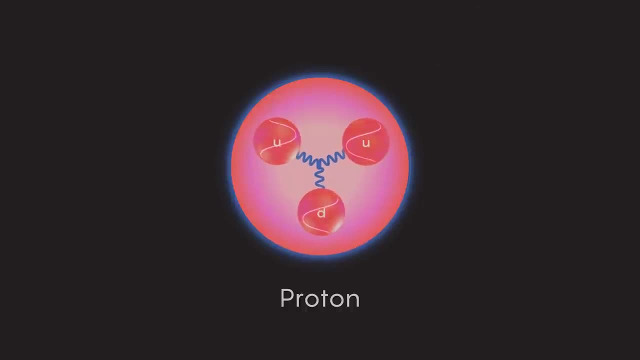 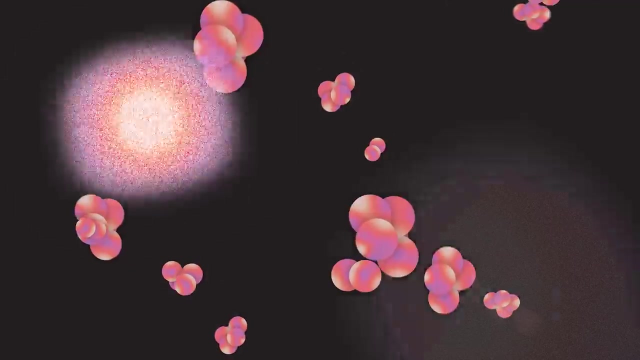 A down quark can turn into an up quark, releasing an electron and a neutrino in the process. This means that a neutron can morph into a proton in what we call radioactive beta decay. In this way, the weak force is responsible for the nuclear fusion reactions that power the sun. 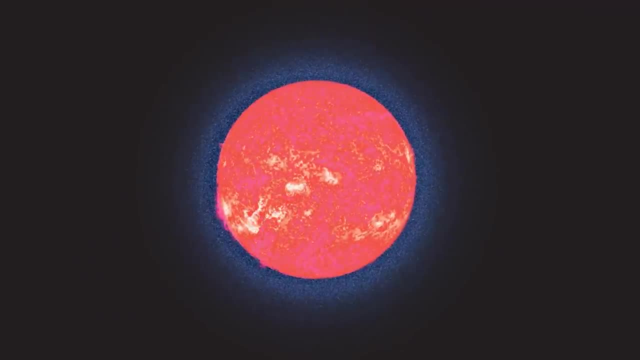 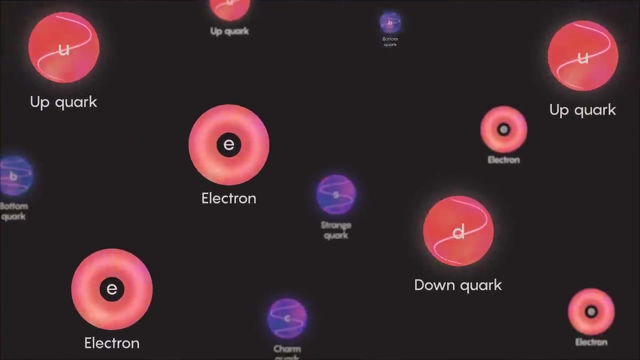 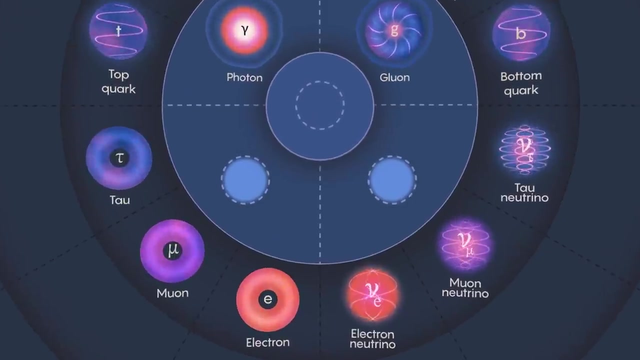 and produce the energy required for life on earth. Finally, the weak force is also the reason that heavier matter particles quickly decay into the three lighter and more stable fermions that make up matter as we know it. There are particles associated to the weak force, and we call these the W and Z bosons. 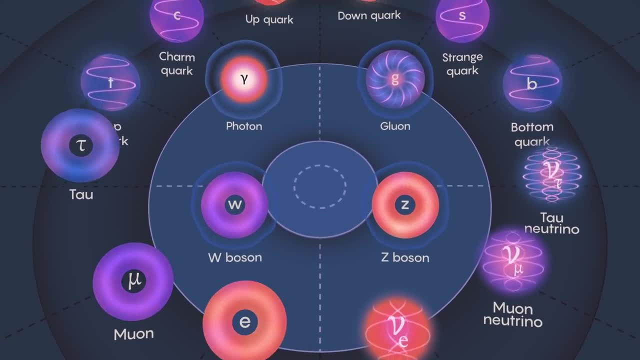 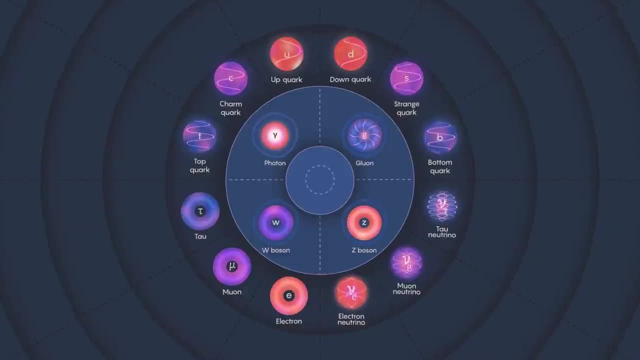 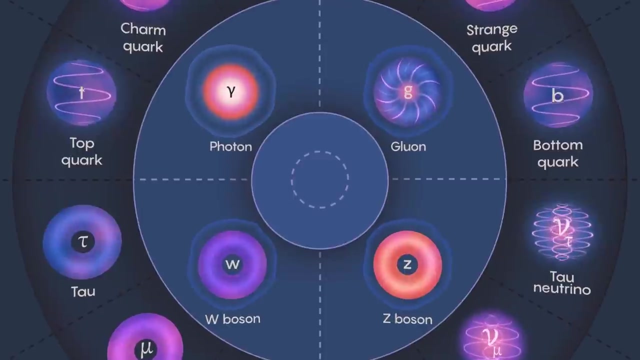 The weak force is the only one of the three forces to act on all particles. In particular, it's the only force that neutrinos feel. Finally, it's time to meet the last piece of the jigsaw, The particle that in many ways, ties the whole standard model together. 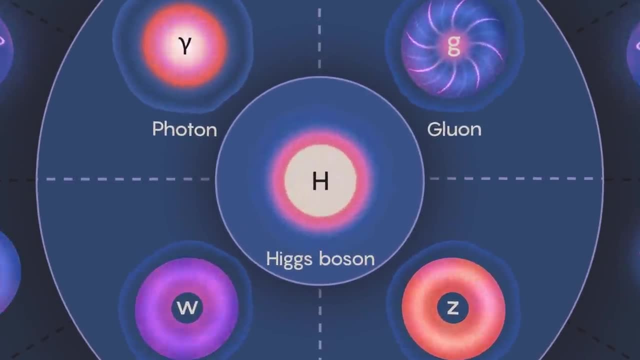 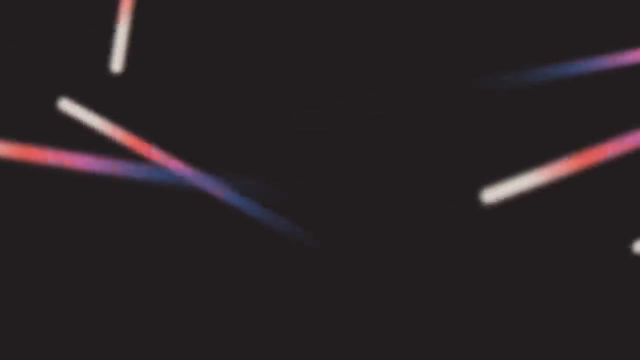 This is the Higgs boson. To explain why the Higgs boson is so special, I should first tell you a striking fact Here: it is None of the fundamental particles in the world have a mass. This is where the Higgs boson comes in. Its role is to endow all fermions with a mass. I'd love to be able to give you a clear explanation for why this happens, But sadly it's difficult to come up with good analogies for the Higgs field. Here's what I would say is a so-so analogy. 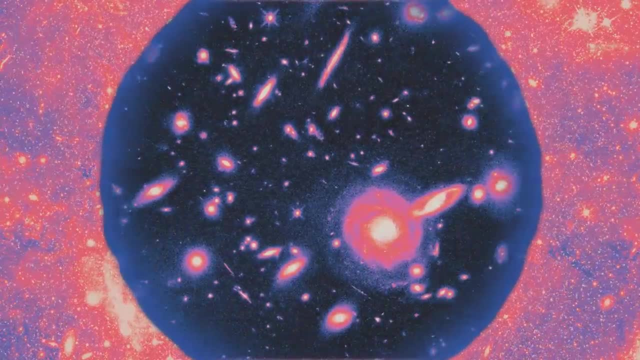 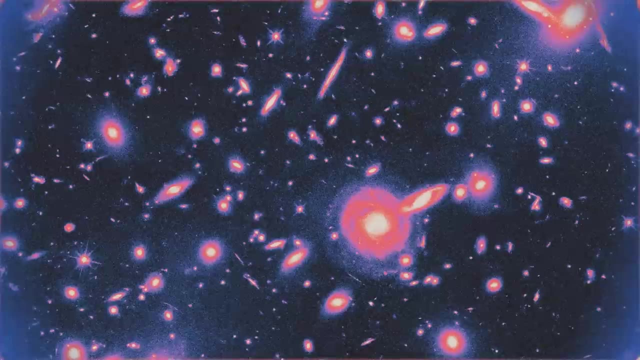 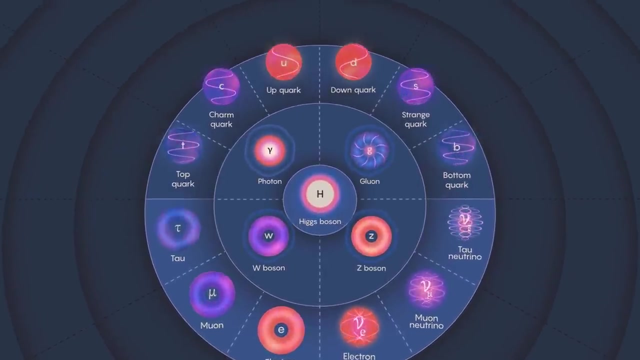 You should view the Higgs field as something like a cosmic molasses Spread throughout the universe, trapping matter particles as they travel through space and giving them what appears to us to be a mass. So this is the standard model: Twelve matter particles interacting with three forces and a Higgs field. 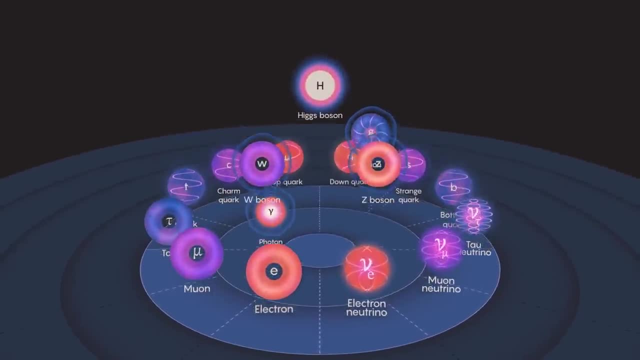 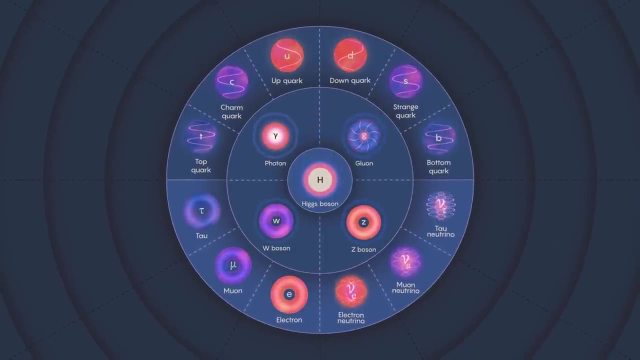 It's a beautiful picture, the pinnacle of 400 years of science, But it's clear that the standard model is not the last word in physics Since the discovery of the Higgs boson. physicists like me feel that in many ways the standard model is too successful. 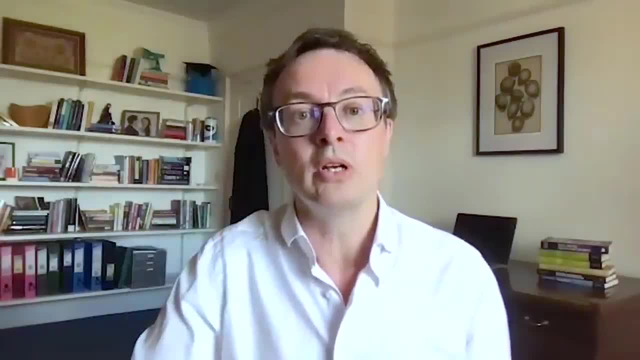 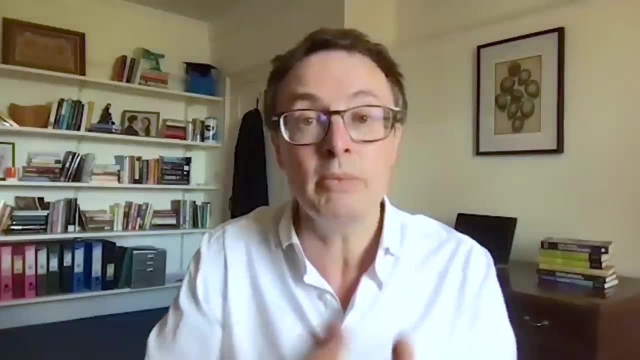 It gives the right answer to every experiment that we do. Our current hope is that we'll eventually find an experiment that it gives the wrong answer to- And there are some hints that this is happening- Because only then can we get clues about what lies beyond. 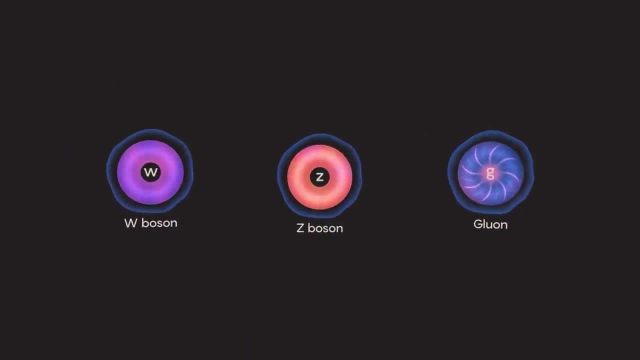 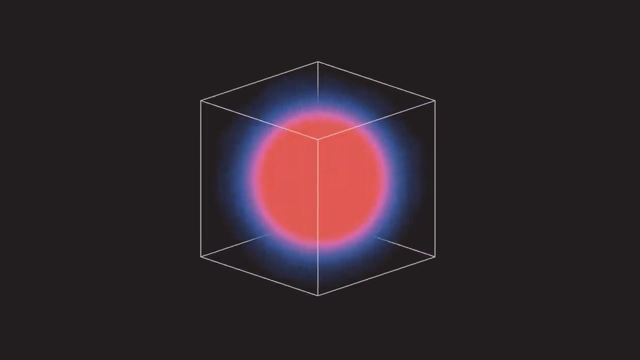 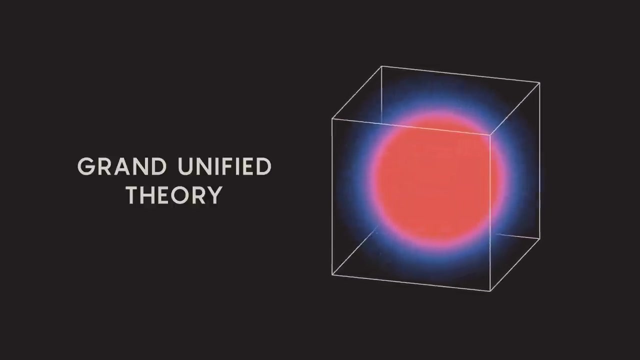 One of the open questions about the standard model is whether the three fundamental forces are actually different or whether they are a manifestation of a single, all-encompassing force. This is the dream of a grand, unified theory. There are some theoretical signs that this may be the way things work out. 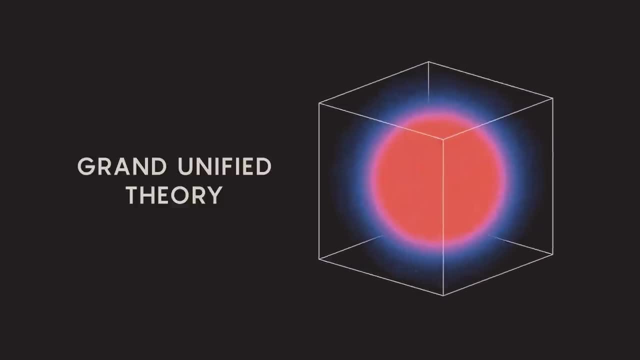 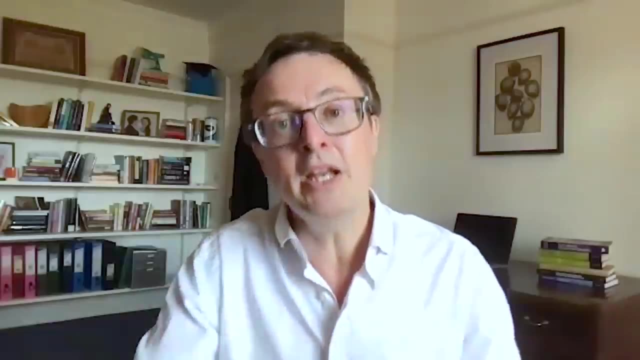 But so far no experimental confirmation. Of course, we're also left with the obvious thing that's missing, And that's gravity. At the beginning of this video, I talked about the problem of quantum gravity. In recent years, we've discovered gravitational waves. 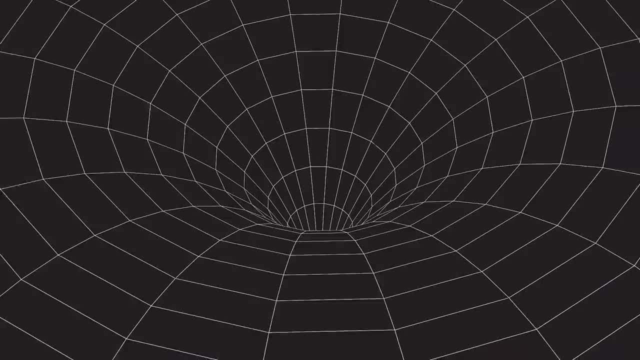 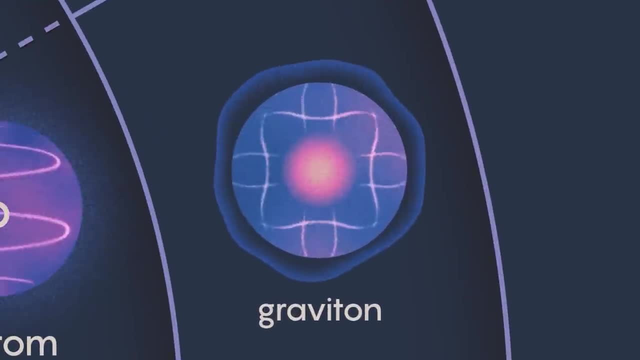 which are ripples of space and time itself. And if we look closely, there are good reasons to believe that these waves are made of quantum particles that we call gravitons, just like light waves are made of photons. There are other things missing too.